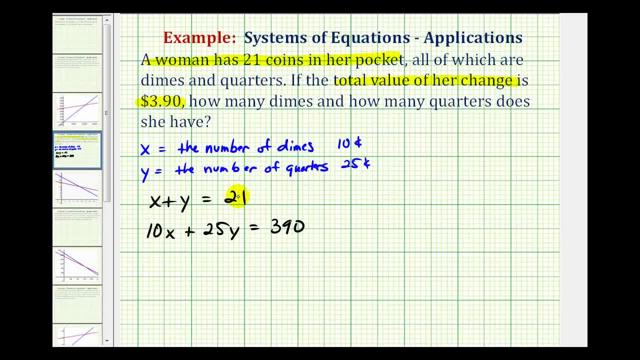 negative ten x. So what we'll do is multiply the first equation by negative ten, then leave the second equation the same. So we're going to multiply this entire equation by negative ten. That's going to give us negative ten x minus ten y. 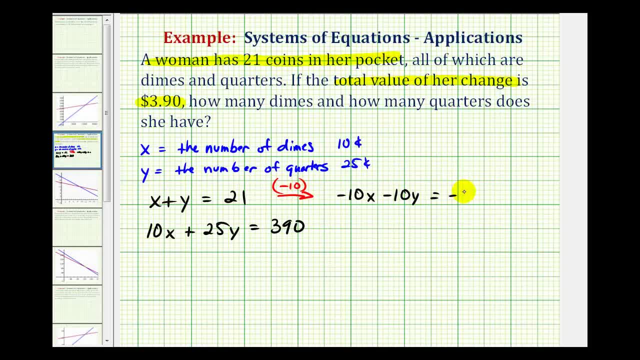 equals twenty-one times negative. ten would be negative two hundred ten. We'll leave the second equation the same. So we have ten x plus twenty-five y equals three hundred and ninety. and then when we add these equations together, since the x terms are opposites, this sum would be zero. 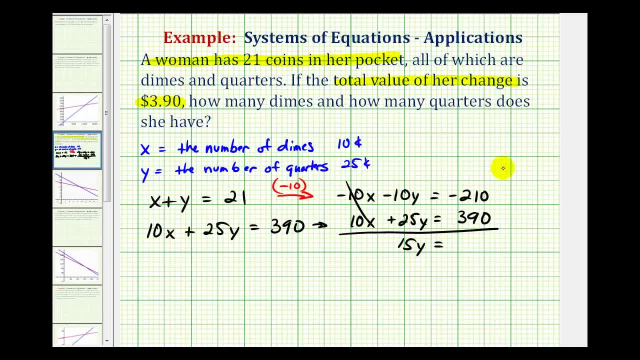 So we'll left with fifteen. y must equal negative two hundred ten plus three hundred ninety, which is equal to one hundred eighty. Now we'll divide both sides by fifteen, and so we have: y equals one hundred eighty divided by fifteen is equal to twelve. 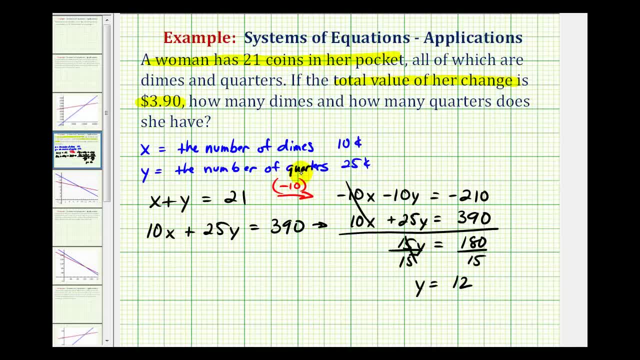 And since y is equal to twelve, this means we have 12 quarters. and now we have to determine how many dimes we have. So we can use the equation x plus y equals 21 and substitute 12 for y, So we'd have x plus 12. 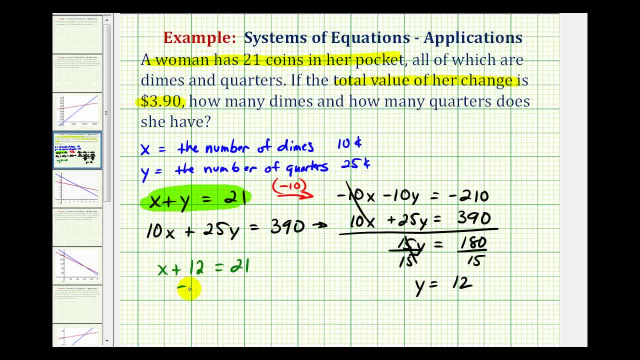 equals 21.. Subtract 12 on both sides, So we have x equals 9.. So this tells us we have nine dimes And twelve quarters. Notice how this gives us 21 coins And nine times ten cents, plus twelve times twenty-five cents. 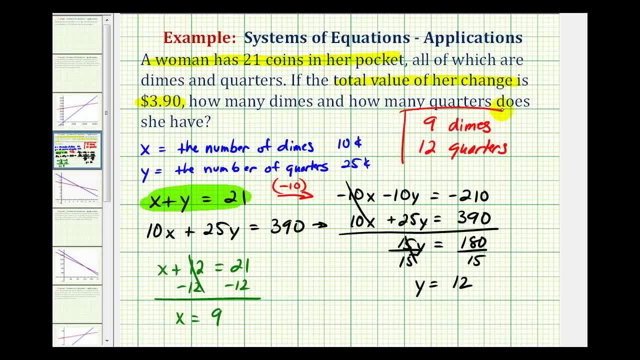 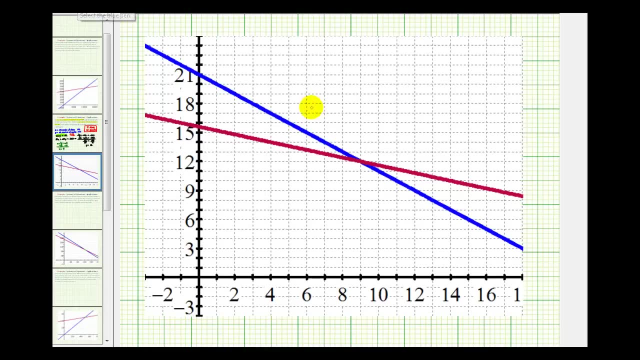 would give us a total of three dollars and ninety cents. Now let's also verify this graphically. Remember: if we graph these two linear equations on the same coordinate plane, the point of intersection would represent the solution. So here's the equation: x plus y equals 21,. and here's the equation 10x.